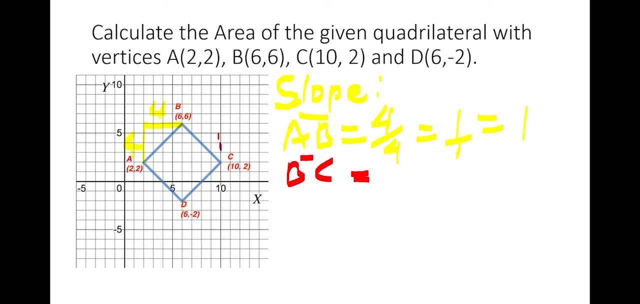 BC, BC, BC, Going up 4 and left 4.. So it's negative 4.. So BC is, rise is 4, run is negative 4.. So it's 1 over negative 1, which is negative 1.. 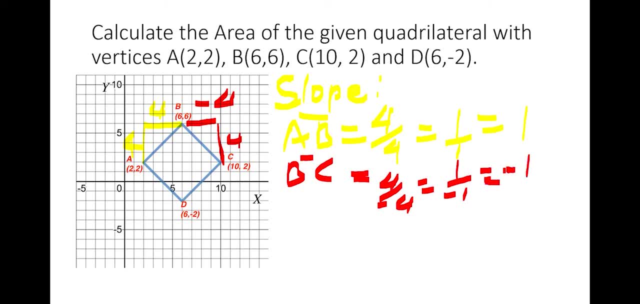 Side BC, BC, Going down, 4, right, Left, 4. Down, 4. Left, 4. Down, 4. Left, 4.. Which is 1 over 1, which is 1.. And then we find side AD. 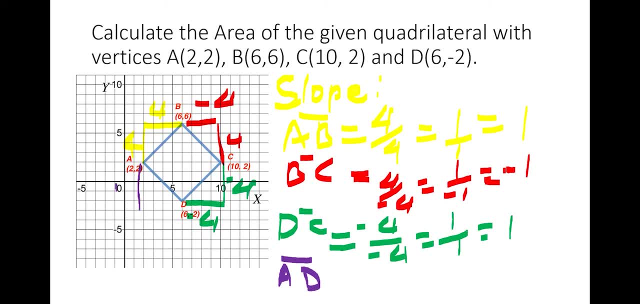 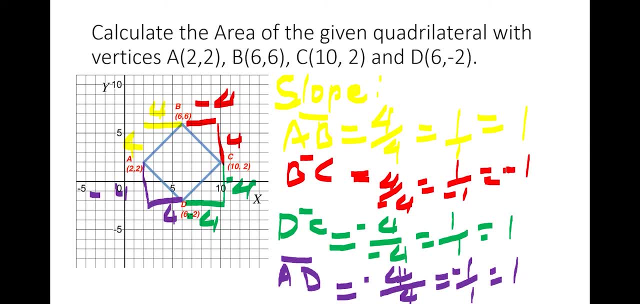 Now let's see What do you see here And what do you notice here When I have: the two sides are perpendicular. First of all, these two sides are perpendicular, These two are perpendicular, They are perpendicular and these two are perpendicular. 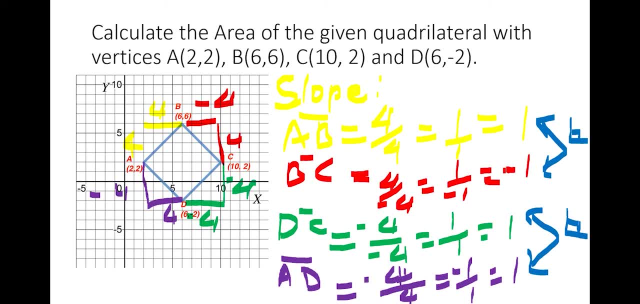 You can see here Deformed 90 degrees, And then we can say: You can see here It's a very firm bar. BC is also perpendicular to DC and a B is also perpendicular to ad right. so these are perpendicular, they form 90 degree. the slope is negative, reciprocal of each other, so 90. 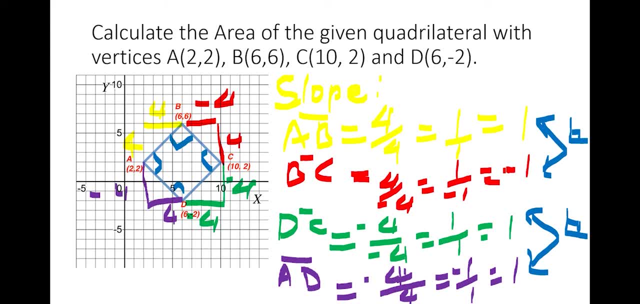 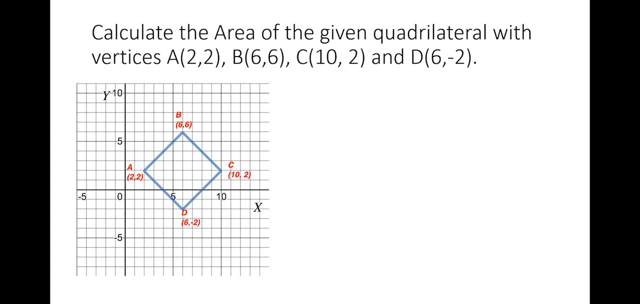 degrees, so this is a square. now in our previous slide we saw that the sides are perpendicular, so the correlator besides from 90 degree. now we have to find the sides, each side land, to make sure it's all the sides are equal and it is a square. so let's start with bt. so our rise was 4 and was 4, so we need to find c. right, we know. 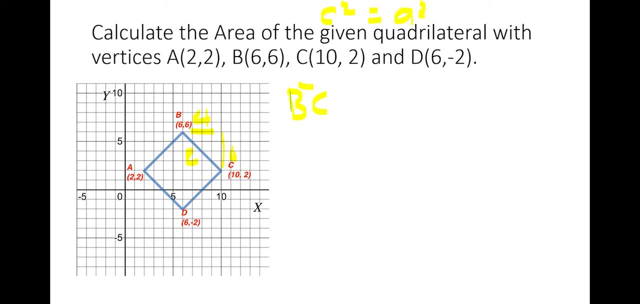 c squared equals a squared plus b squared. right to find c, we'll take square root of a squared plus b squared. so now you're going to take square root of 4 squared plus 4 squared. we know 4 squared is 16, so 16 plus 16 is square root of 32. so square root of 32 is not a perfect square. we leave it. 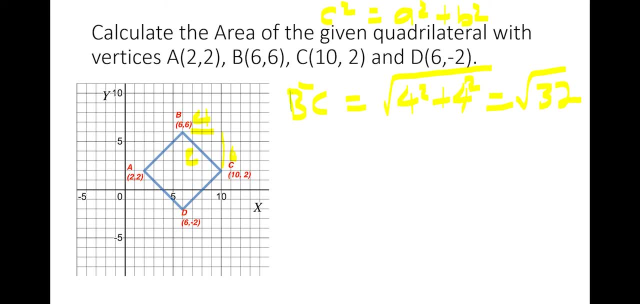 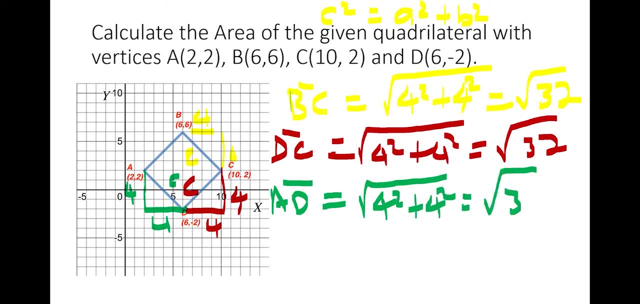 plus 4 squared, which is square root of 32 again. and then we have to find: side a b is 4 and 4, so this is our c. so side a b is 4 squared plus 4 squared, which is square root of 32.